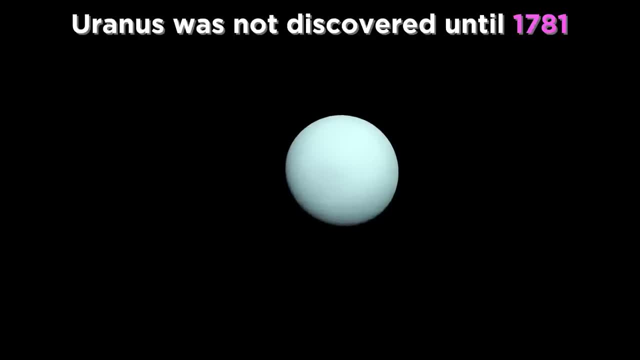 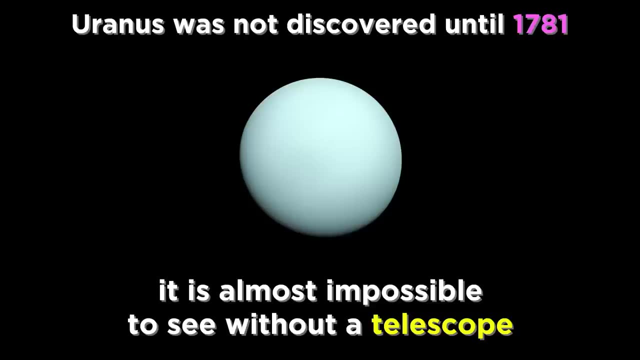 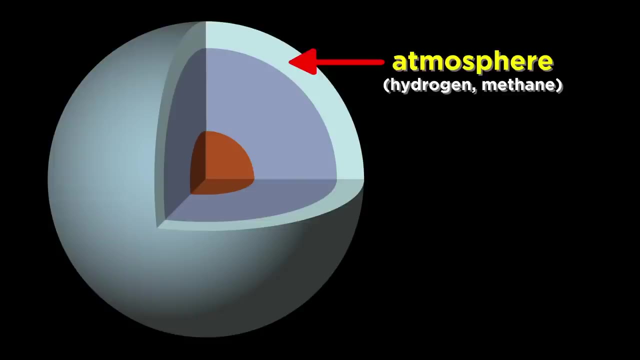 four times that of Earth's. The smaller size, combined with the incredible distance, explains why this planet was never seen until the age of telescopes, as it is almost invisible to the naked eye. Similar to the other gas giants, Uranus has an atmosphere rich in hydrogen and also lots. 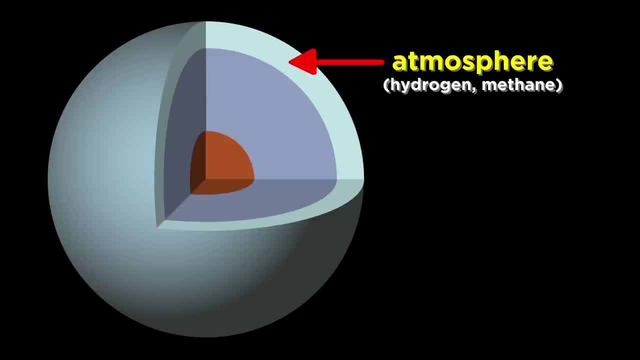 of methane, and it is the methane that gives the planet its deep blue color. Its interior is different from that of the larger gas giants, with no metallic hydrogen to be found From assessing density. Uranus is thought to be a layer of hydrogen gas surrounding. 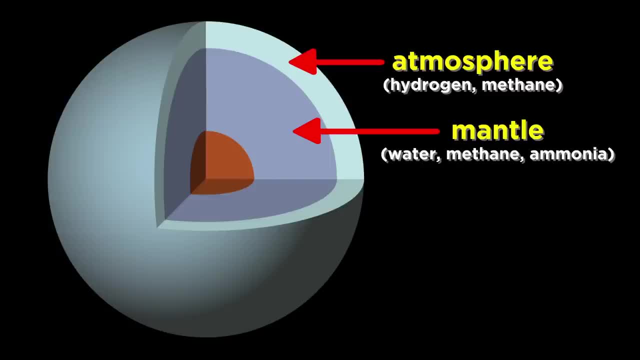 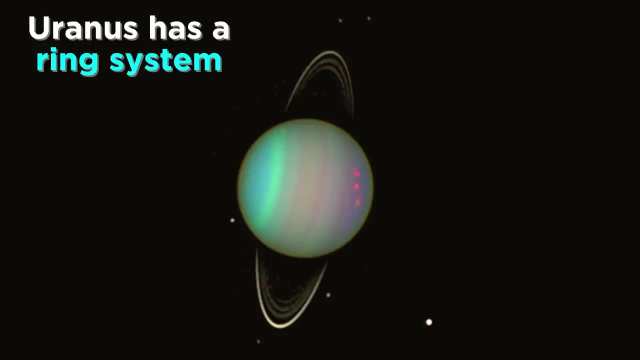 a layer of water mixed with methane and ammonia and with a core of iron and rock. Uranus has a system of rings just like Saturn, with a very similar distribution, though not quite as complex. They are likely to be very icy, like Saturn's rings. 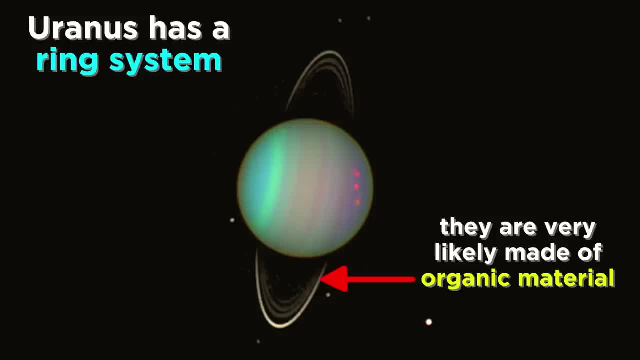 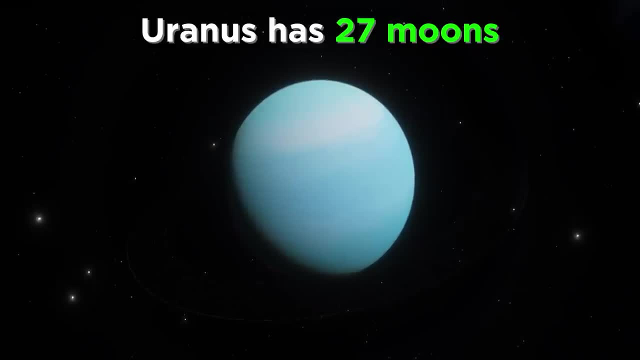 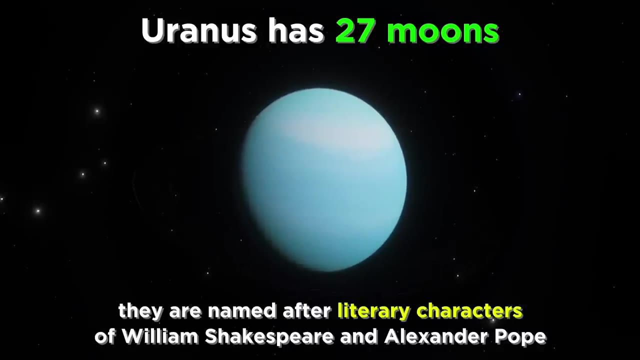 Instead, they are more likely to be comprised of organic material. Uranus also has an extensive system of moons, twenty-seven of them to be exact, and five of them are large. All of the moons are named after literary characters of William Shakespeare and Alexander. 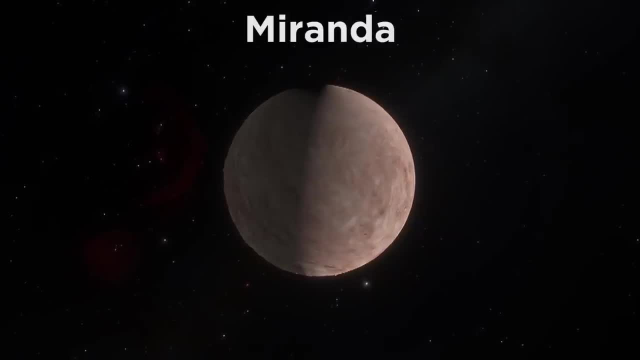 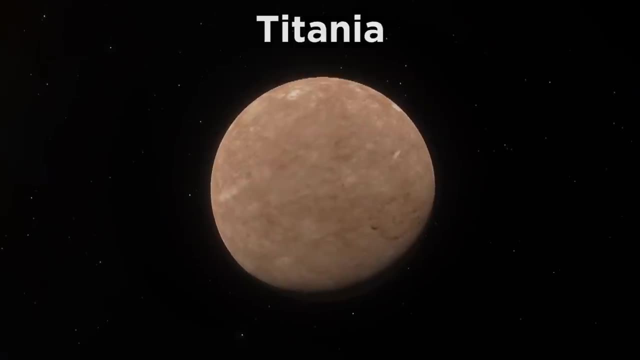 Pope, with the five big ones being Miranda, Ariel, Umbriel and Juliet. Like all the other moons in the world, the Great Sun does have a very large, rich atmosphere. They all end up in the same cone: titania and oberon. 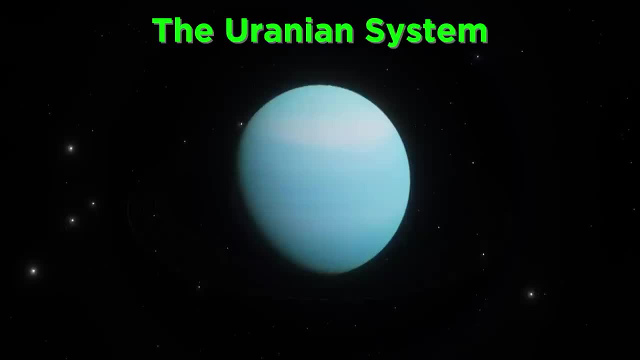 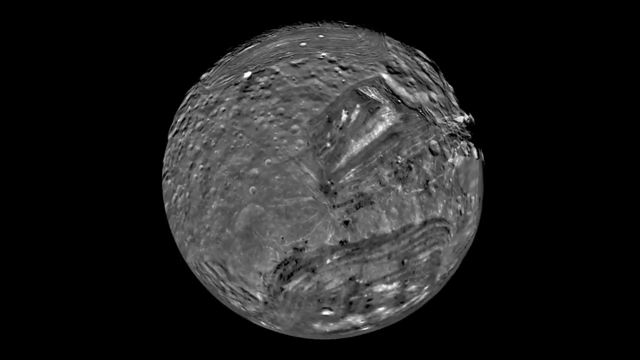 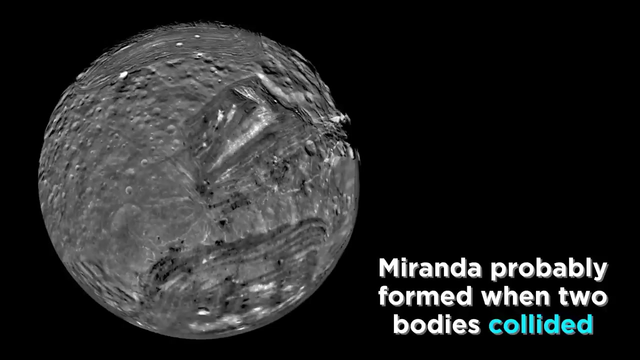 They form a system, just like the moons of the other gas giants, and they are comprised of ice and rock. The smallest of these five moons, Miranda, has a bizarre patchwork appearance, broken into distinct areas that are seemingly unrelated. This suggests that the moon formed as the result of a collision between two separate 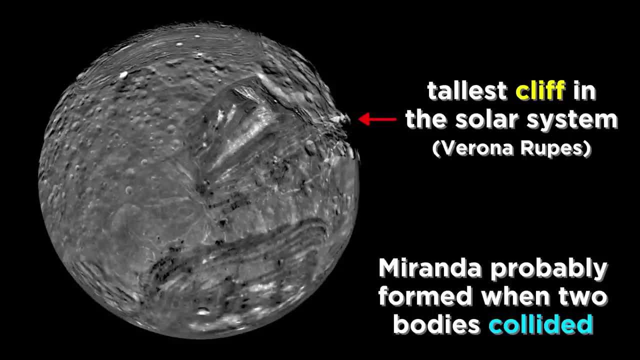 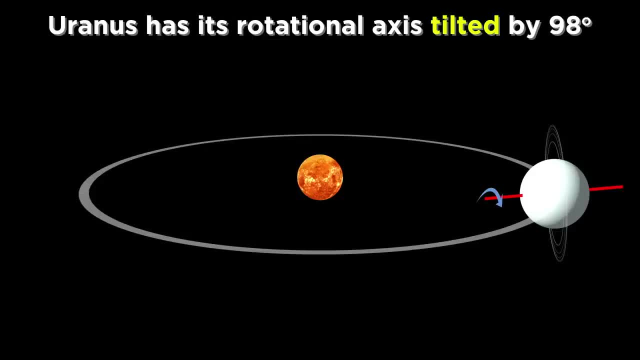 bodies that then merged to form one moon, leaving behind enormous cliffs twice the height of Mount Everest. One peculiar feature of Uranus is its extreme tilt, with its equatorial plane nearly perpendicular to the plane of its orbit. This means that one hemisphere gets daytime for half the year, while the other is in perpetual.